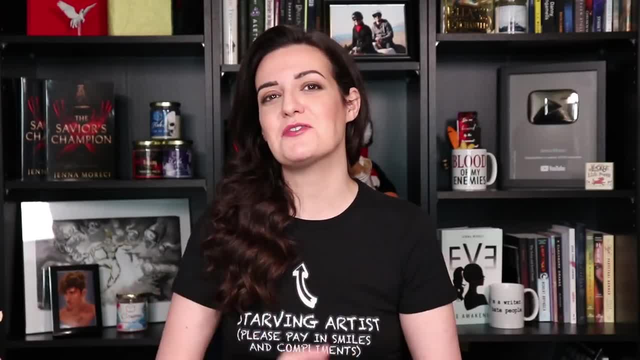 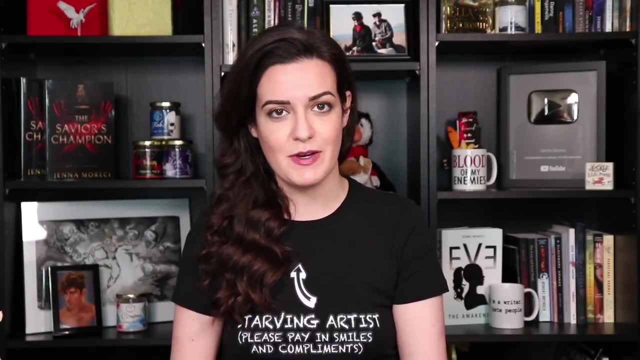 to demystify moral grayness, so you can write yourself a bunch of shady-ass characters. First things first, I want to give a shout out to Audible, who has generously sponsored today's video. You guys already know about Audible, I'm sure, but if you're not familiar, they feature. 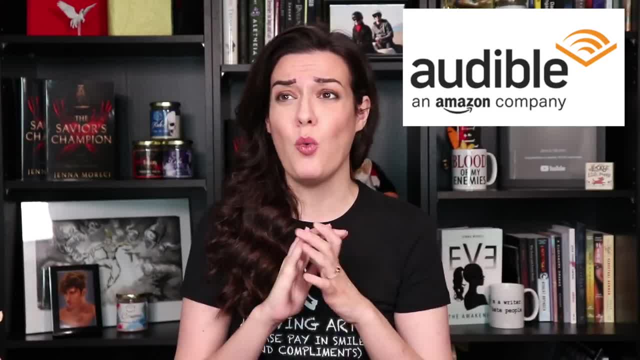 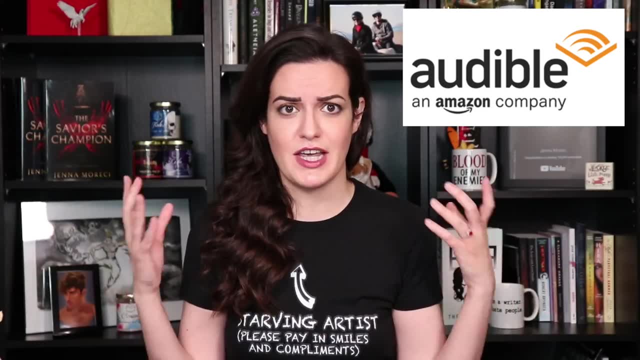 an unmatched selection of books. I'm sure you're familiar with Audible, but if you're not familiar, they have audiobooks in a wide variety of genres like fantasy, sci-fi, romance and a TON of other selections like news and comedy. On top of that, they have Audible Originals, which are exclusive. 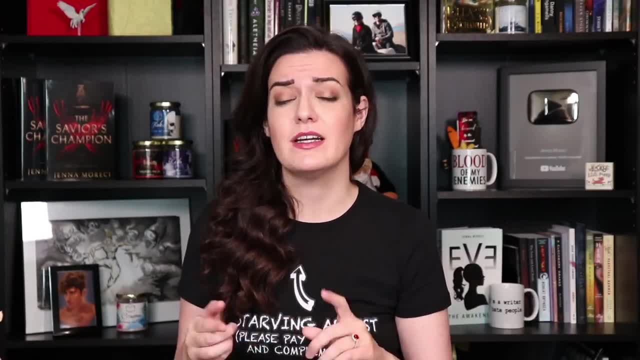 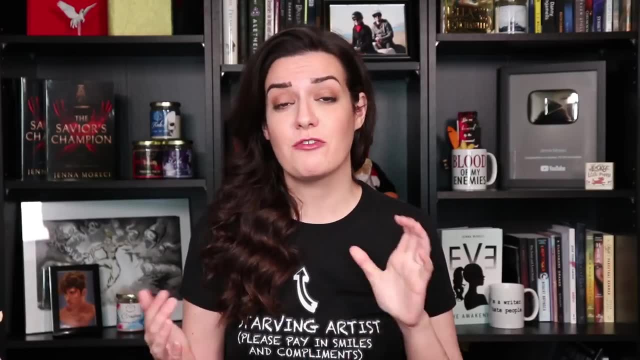 audio titles created by celebrated storytellers in literature, theater, journalism and so on. You can get the Audible app for free on your phone or your tablet. I personally like having it on my phone because then I can listen to audiobooks and I don't have to worry about. 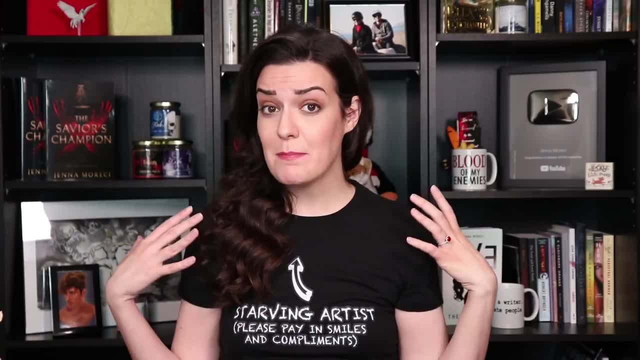 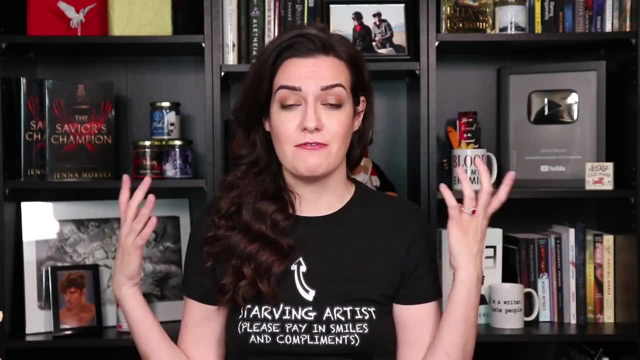 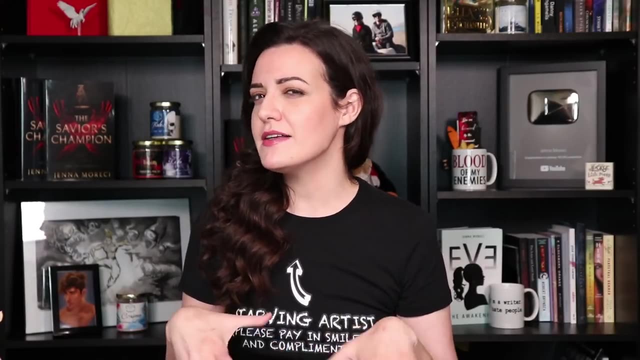 audiobooks while I'm cooking or while I'm doing chores. They also have a bunch of membership perks, like one free audiobook a month, exclusive sales and 30% off all regularly priced audiobooks. If you're interested in checking out audiobooks featuring morally gray characters, might I? 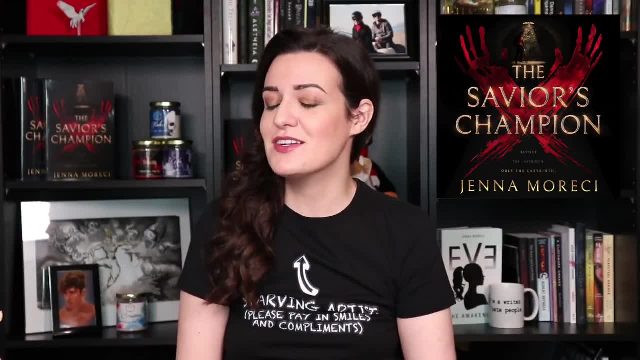 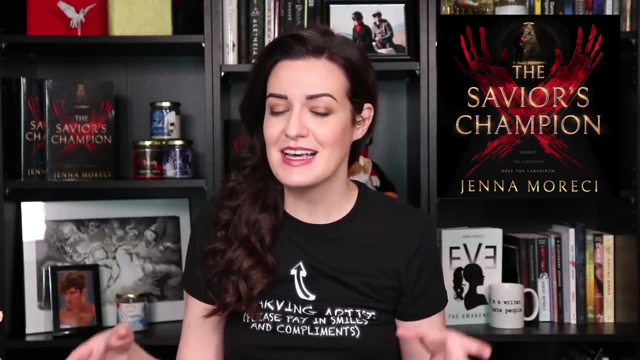 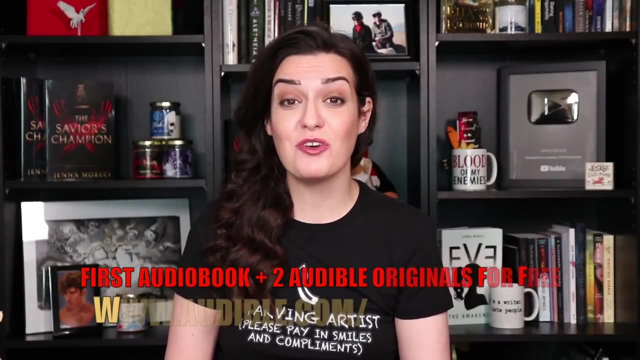 suggest The Savior's Champion. It's a dark fantasy novel with a massive cast, most of whom are morally gray. So if you like violence and romance, give it a listen on Audible and I'll see you next time. I have it on good authority that it's the tits. Even better, you can get your first audiobook for 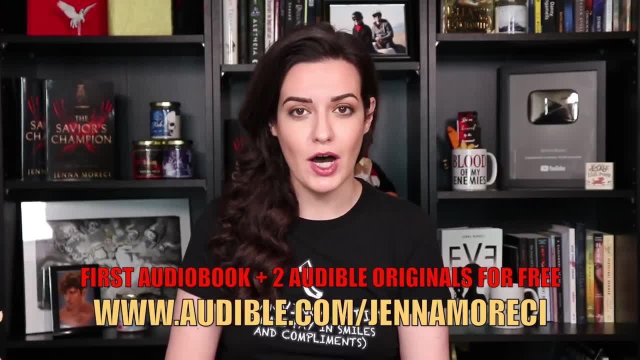 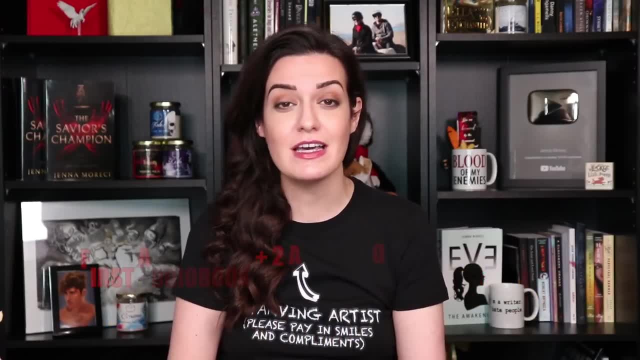 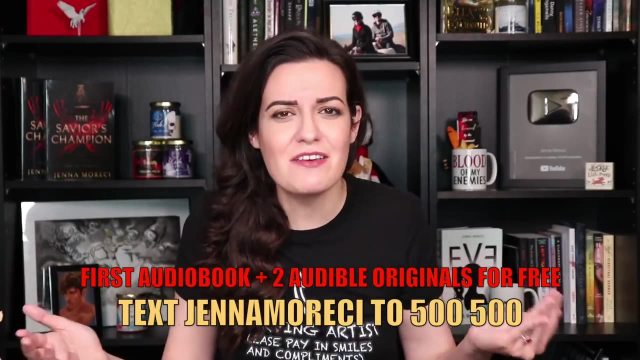 free plus two Audible Originals when you try out Audible for 30 days. All you have to do is visit audiblecom, slash Jenna Moreci or text Jenna Moreci to 500500.. And you know that free audiobook can be The Savior's Champion. It's got a love story, It's got bloodshed, It's got morally gray characters. 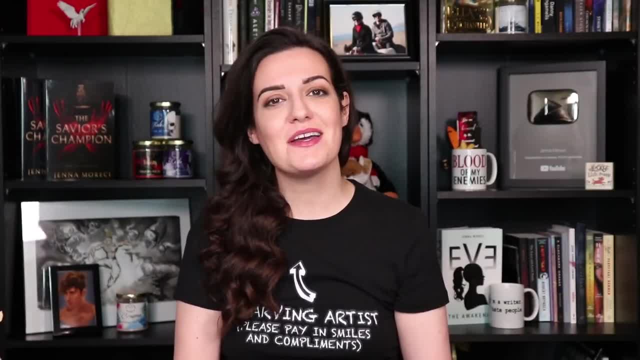 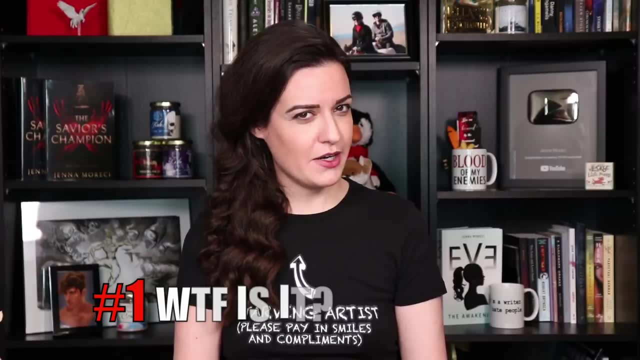 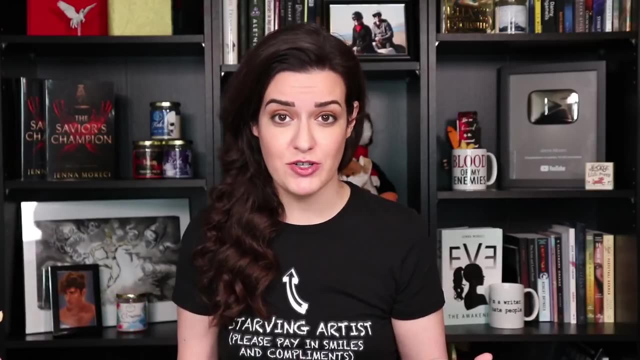 What more could you ask for? Onto the topic, We are breaking down the mystery that is the morally gray character in three, two, one go. What is a morally gray character? A morally gray character is a character who is morally ambiguous. They've got good traits and bad traits. They do good things. 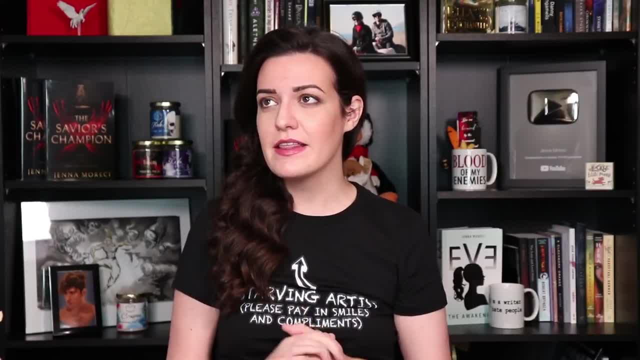 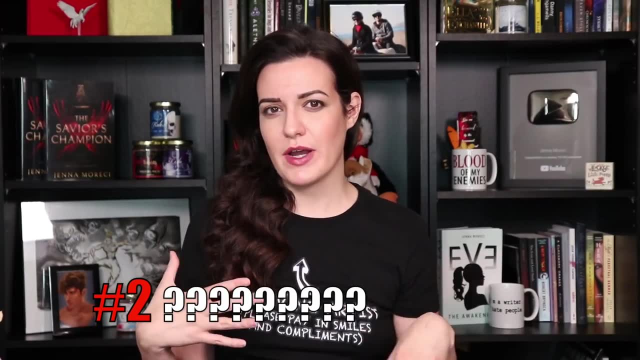 and bad things. One moment they may seem like the good guy, the next moment they may seem kind of evil. Why is this concept so confusing? While the definition of morally gray character is a character who may seem straightforward, it kinda isn't. No one can seem to agree on how heavily we 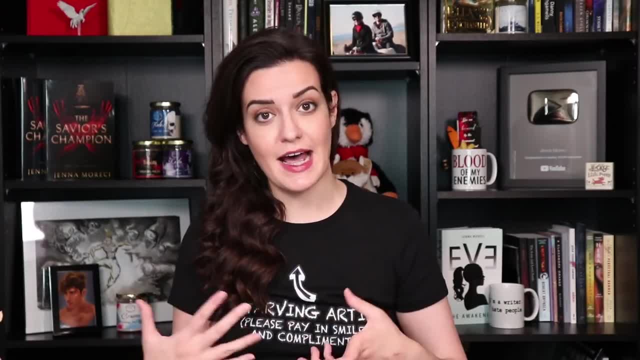 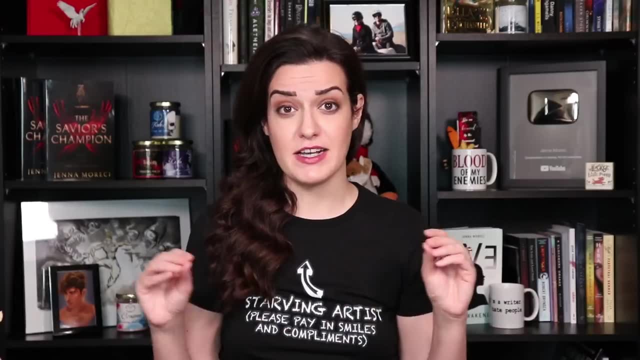 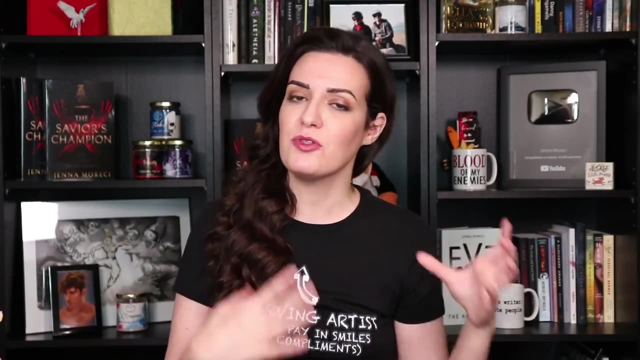 can read into the definition or what additives we can tack on to it. There are a few schools of thoughts involving morally gray characters, but the two I see most often are as follows. First is the simplest option. Morally gray characters do both good and bad things and have both good. 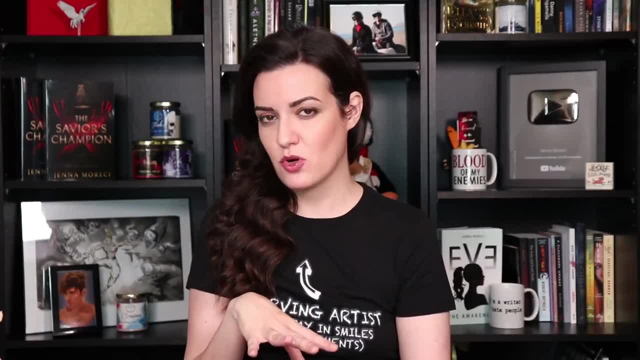 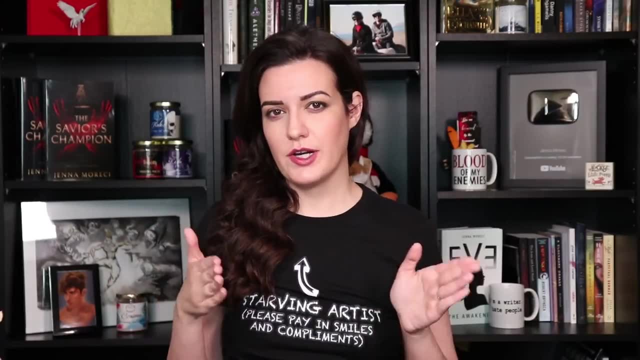 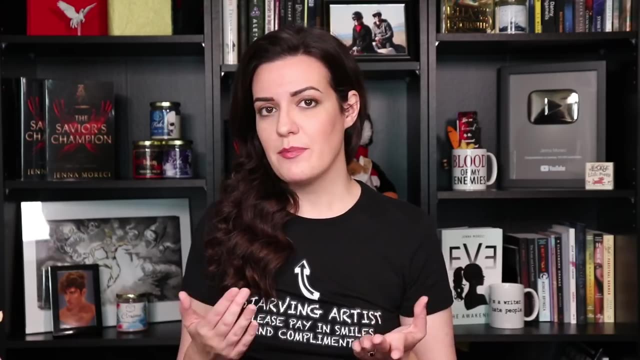 and bad motivations. Looking at this interpretation of moral grayness, a hefty chunk of it is that a lot of characters fit under this label, Whether they lean more so toward being a good guy or a bad guy. a lot of characters do both good and bad things for a variety of impulses. For example, 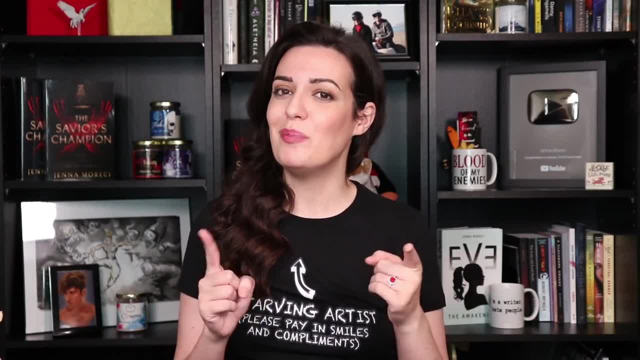 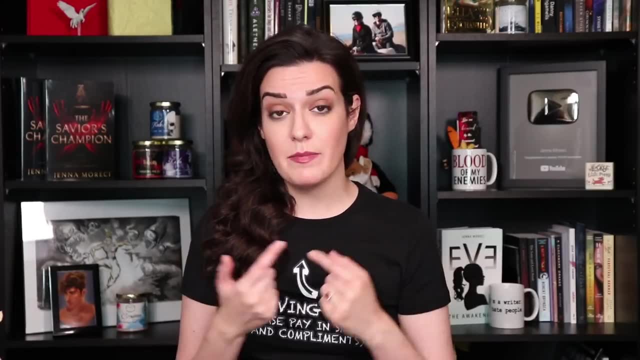 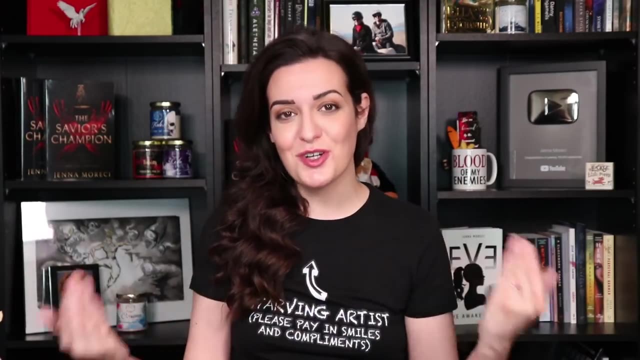 Robin Hood steals from the rich, which is bad, but he gives to the poor, which is good, So he would be considered morally gray. Diving in deeper, we can look at Tobias from The Savior's Champion. His primary motivations are helping his family and protecting his girlfriend, which are good. 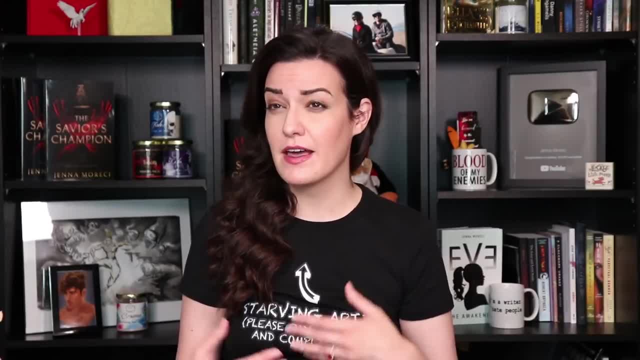 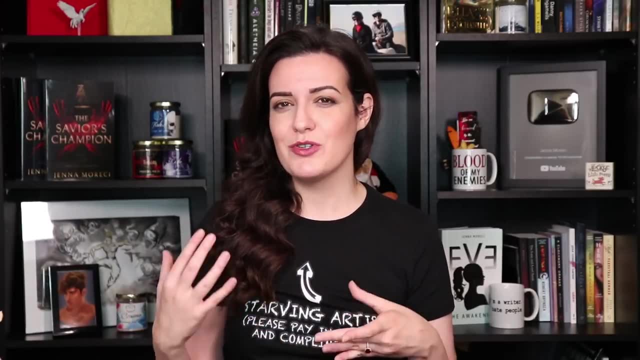 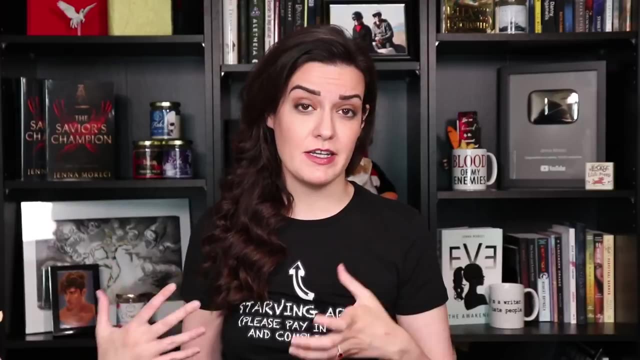 but he also murders and assists in the murder of several people, And while some of those situations are self-defense, most are revenge fueled, which is a bad motivation. Thus, according to this interpretation, Tobias would be seen as morally gray. Then there's the second interpretation. 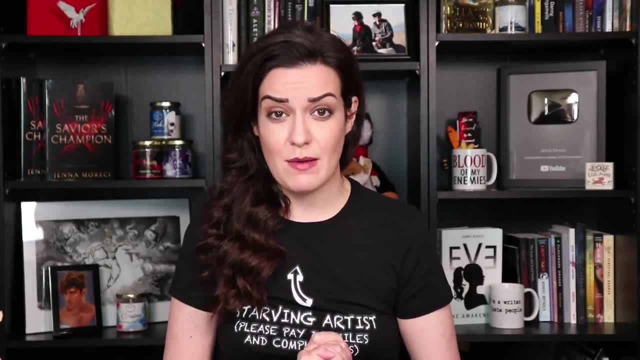 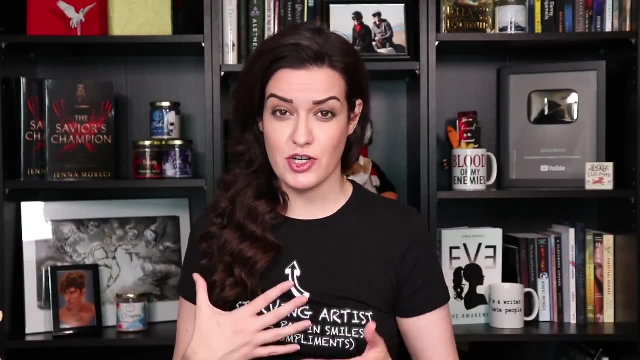 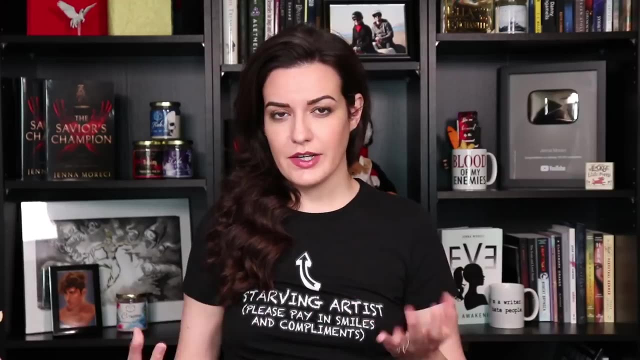 which is a bit more complicated. This school of thought believes that morally gray characters commit both good and bad actions. However, their motivations are hard to determine. In this situation, the lack of clarity is key. Their motivations are unclear or unknown. Looking at Tobias, while he does both good and bad things, his motivations? 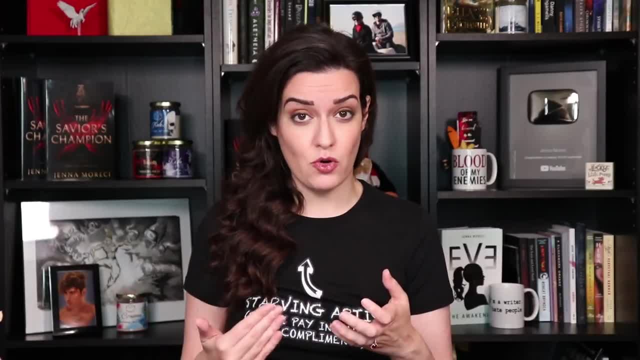 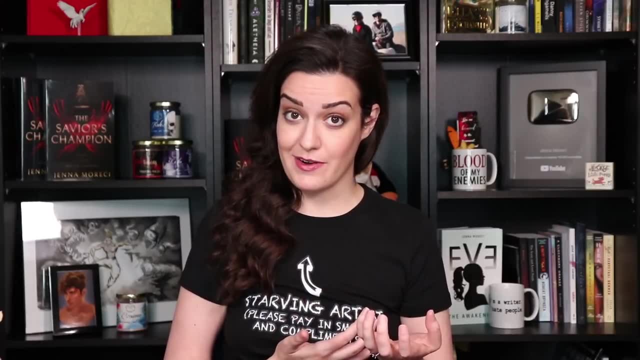 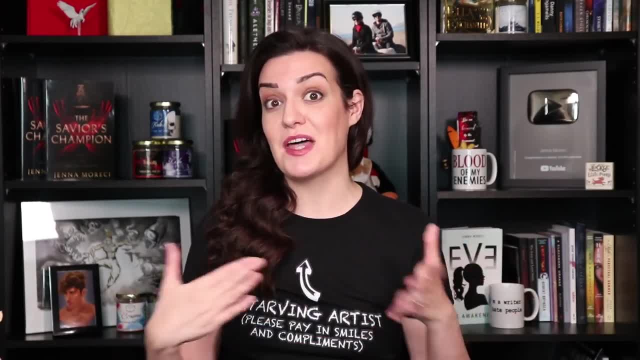 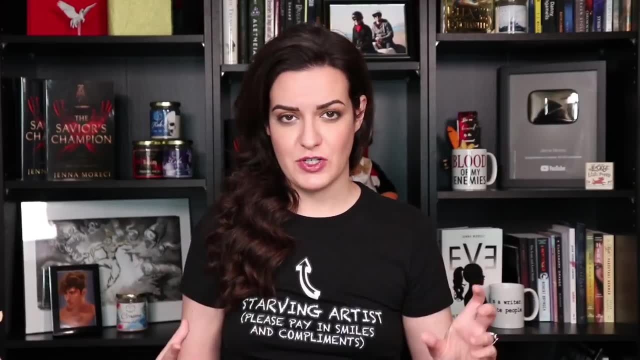 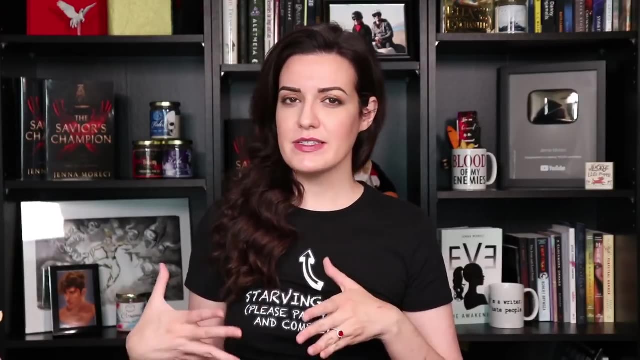 However, I can't really continue on to the next points without picking a side. Thus, I'm going to focus on the interpretation that I believe makes the most sense, and that's the first one. Morally gray characters do good and bad things and have both good and bad motivations. The reason I lead 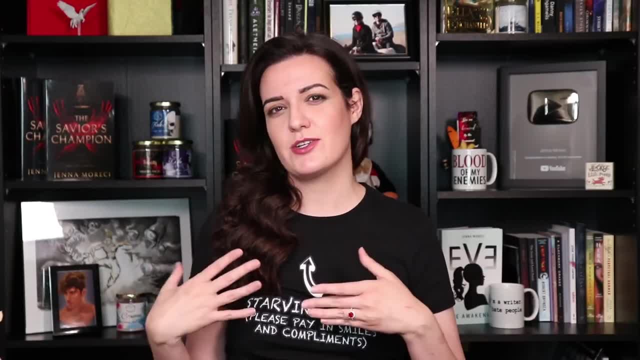 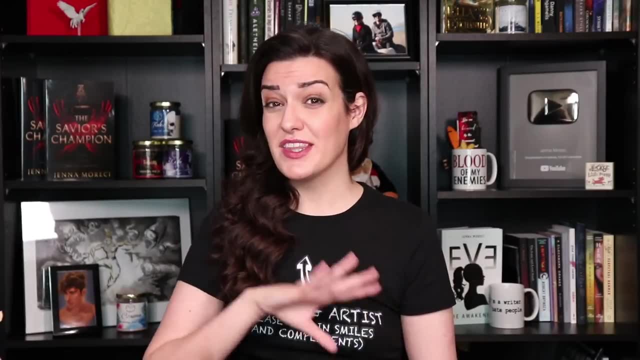 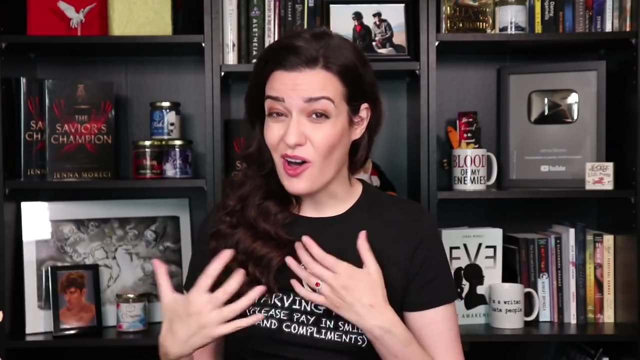 toward this interpretation is: it's pretty common for a character's motivations to be revealed, If not initially, then as the book or series progresses. Thus, if we look at the second interpretation, very few characters would be categorized as morally gray. In fact, all the characters that 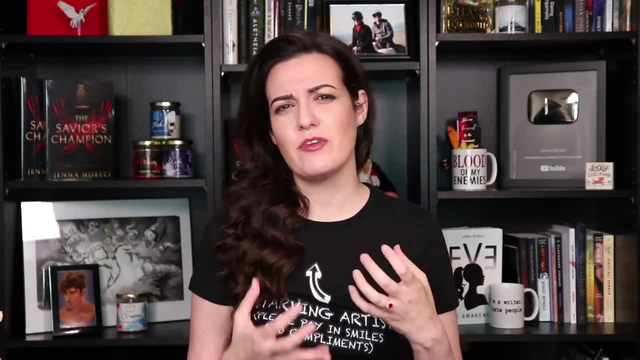 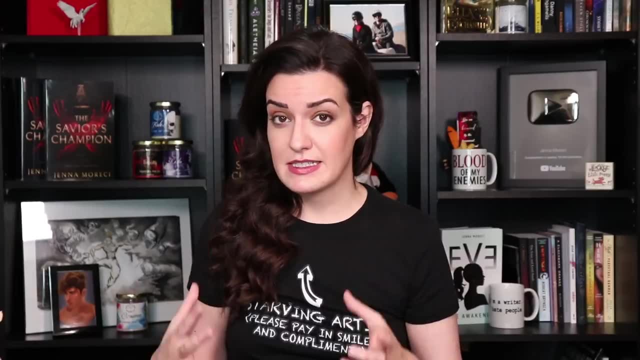 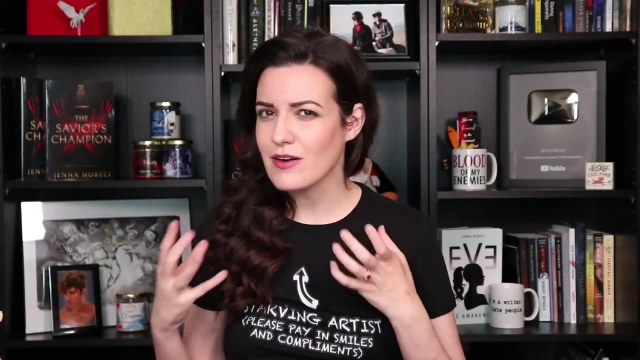 I've seen listed alongside this interpretation, have had their motivations revealed, which directly contradicts the definition. Even if a motivation isn't explicitly stated, it's often showcased through action, emotion or dialogue. So it's kind of hard to keep the reader in the dark forever If a character has both good and bad motivations, and they're not. 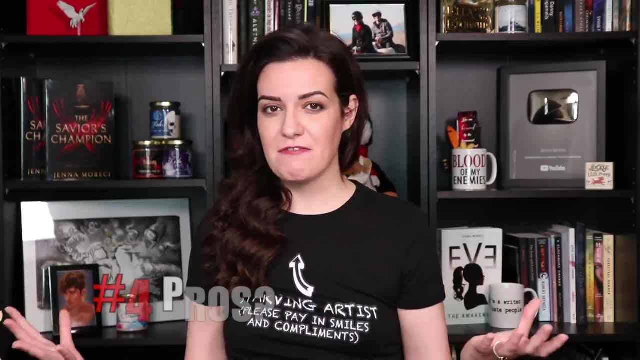 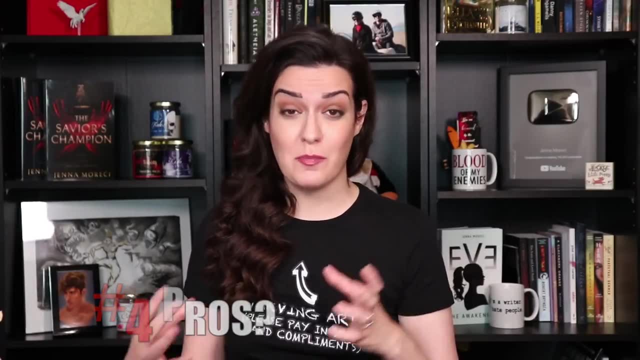 good, then I personally believe they're morally gray. What are the benefits of writing morally gray characters? The biggest benefit is that they're realistic. Most people, even if they're good or bad people, are not 100% pure or 100% evil. I consider myself a good person who is 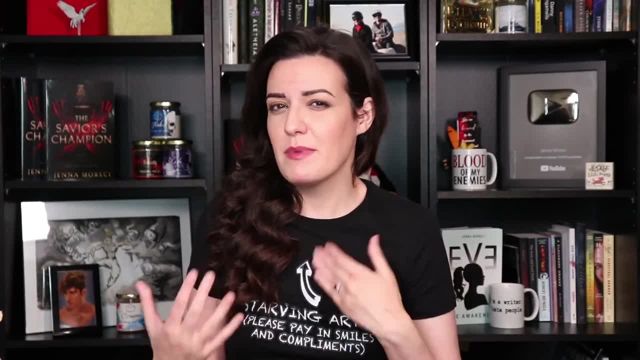 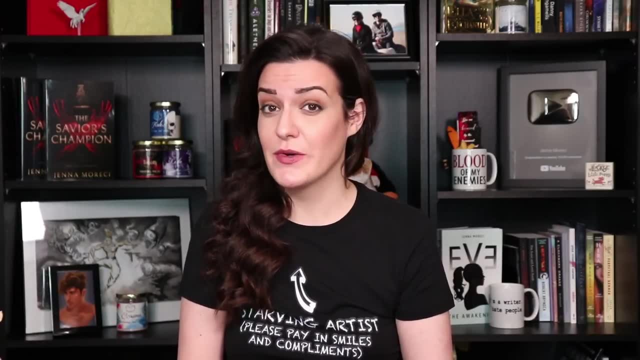 motivated by good, but I've fucked up before and I've made decisions that had some less than pure motivations. Readers tend to find morally gray characters believable because they're inaccurate and often relatable, but I don't think that's the case. I think they're more likely to be. 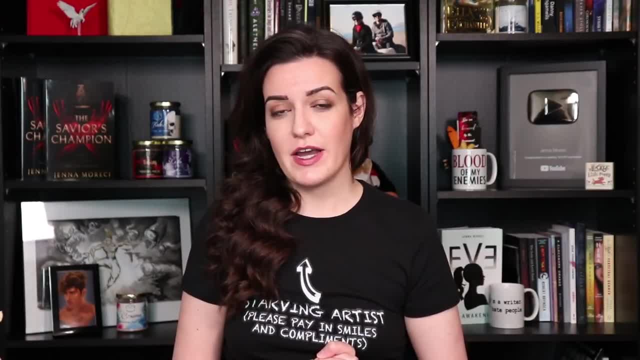 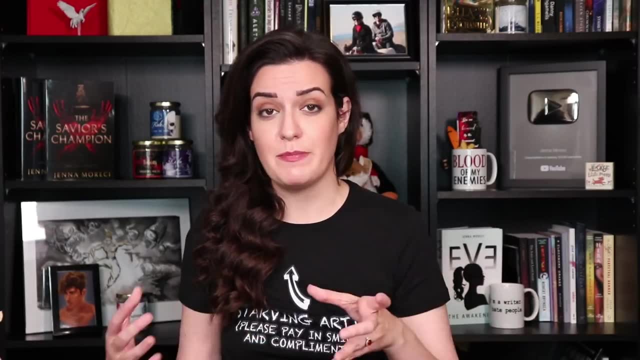 a look into the human experience. The next benefit of morally gray characters is that they are multi-dimensional, which makes them engaging to read. Sometimes, characters who are just good or just bad can come off as flat, because it feels like that's all there is to them. They're. 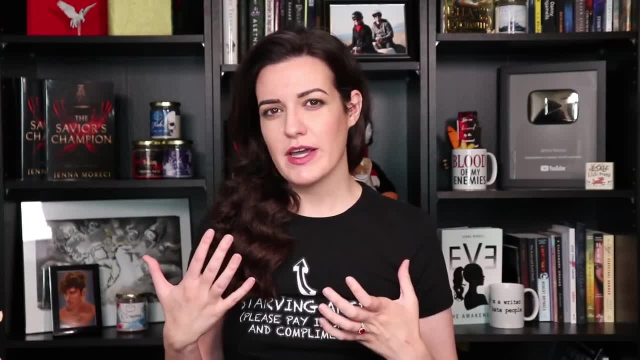 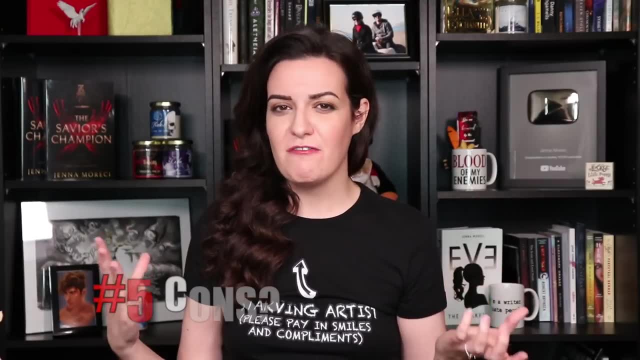 just a hero. They're just evil. Morally gray characters tend to come off a lot more layered, because both their assets and flaws are on full display. What are the pitfalls to writing morally gray characters? The first pitfall is: all of them. Morally gray characters tend to be more. 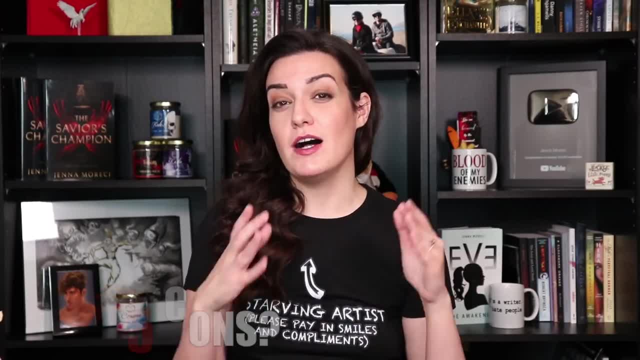 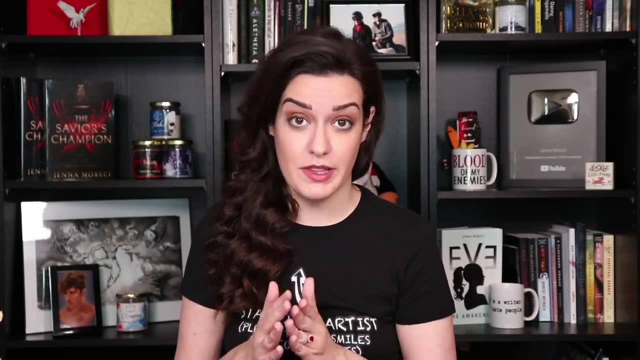 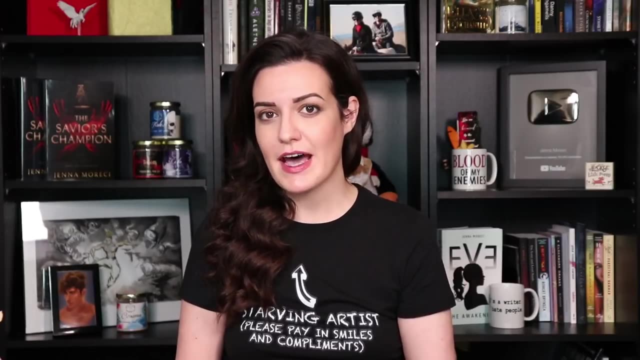 realistic, but also realism. While it's true that most people are not 100% pure or 100% evil, a lot of people lean heavily in one direction or the other. I'm sure you can think of a lot of people throughout history who have done a ton of horrible things. Maybe they had a redeeming. 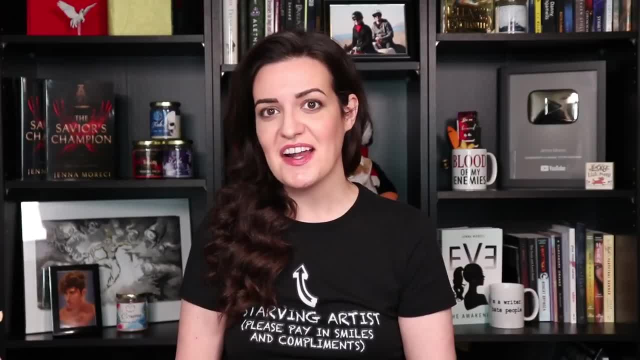 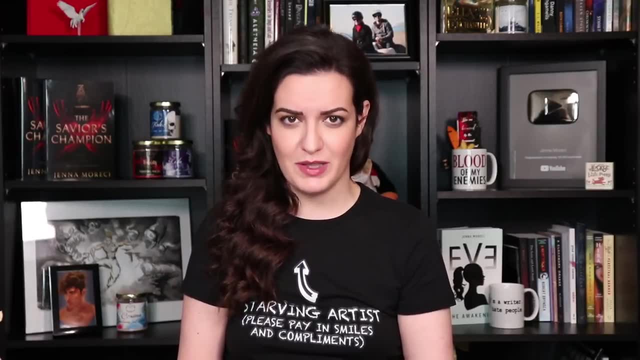 quality or two, but in the midst of prejudice and genocide, that doesn't amount to much. Additionally, there have been people who have devoted their lives to others or making the world a better place. Sometimes people have done a lot more than they should have done, and sometimes they've done. a lot more than they should have done. Sometimes people have done a lot more than they should have done. Sometimes people have done a lot more than they should have done. Sometimes people have done a lot more than they should have done. Sometimes people are genuinely good-natured. 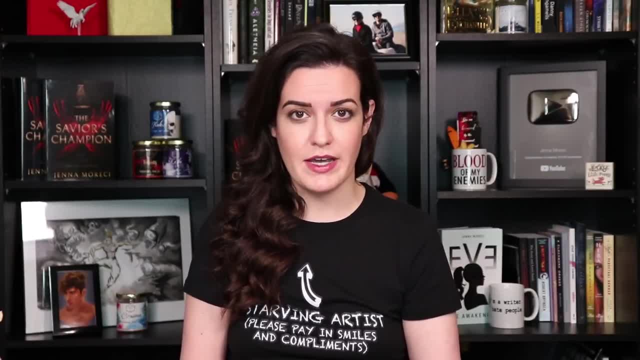 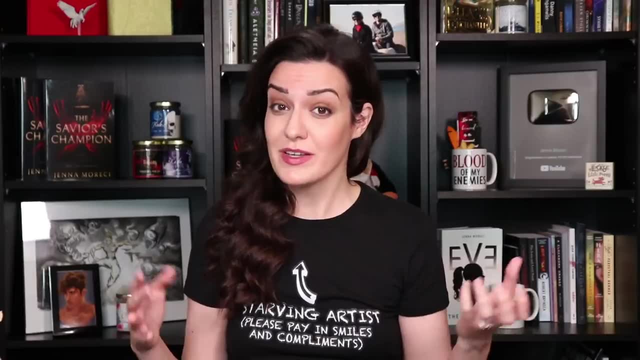 There isn't anything inherently wrong with writing morally gray characters, because they are prevalent, but sprinkling in some evil-doers and good-doers is a smart idea, because they exist too. The second pitfall is the unlikability factor. While not all morally gray characters are, 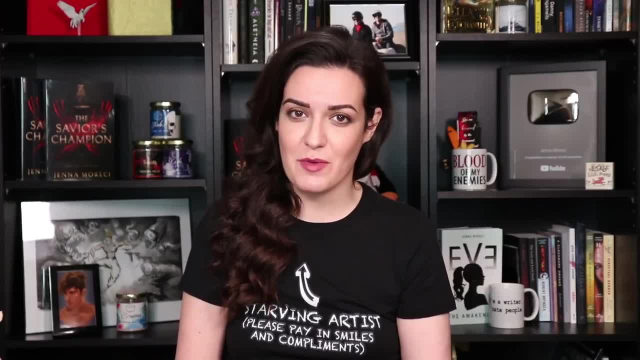 supposed to be likable. many are, especially if they're the protagonist. Problem is when you're juggling both good and bad acts, as well as good and bad motivations, it can be easy to get in the way of what you think is right and what's wrong, But if you're juggling both good. 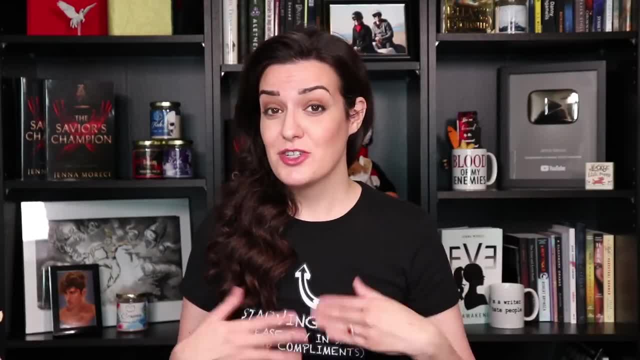 and bad acts, as well as good and bad motivations. it can be easy to get in the way of what you think is wrong, But if you're juggling both good and bad motivations, it can be easy to tip the scales in one direction and turn the audience against the character. There are certain lines that 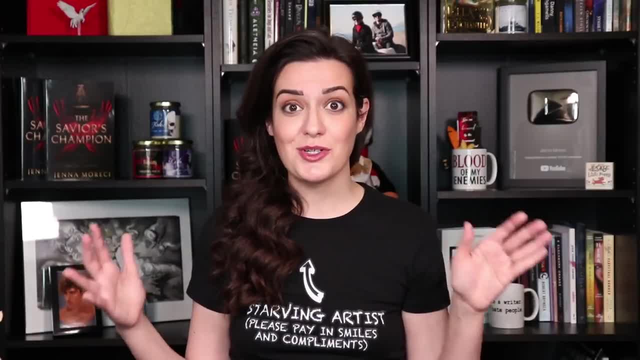 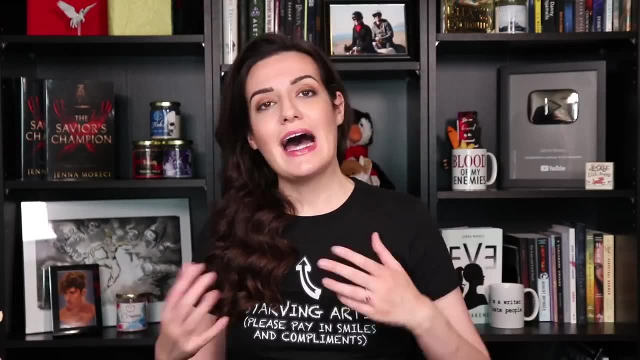 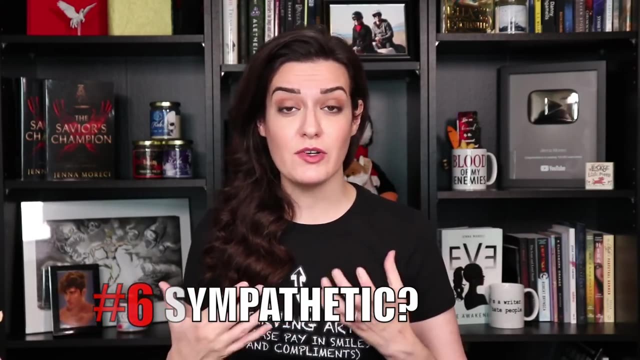 once crossed, there's no going back. The character is now dirt. You have to heavily weigh the justifications of their actions and make sure the audience is on board. How do I write a sympathetic, morally gray character? A sympathetic, morally gray character is basically a morally gray. 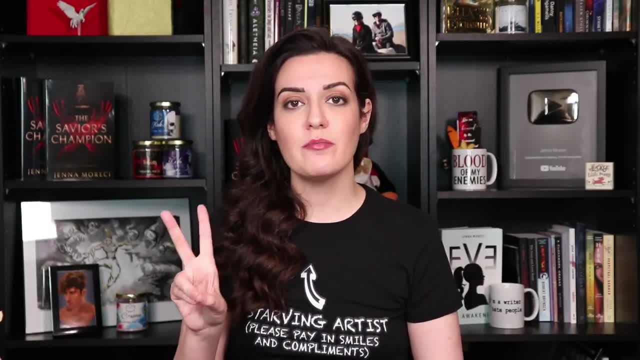 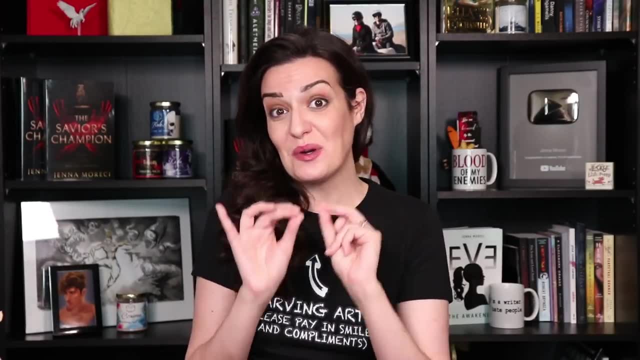 character that readers root for, and there are two components to nailing this. First, your character needs to wrestle with important decisions that could potentially be really bad. If they're perfectly fine with doing something evil, then they're gonna be seen as evil. 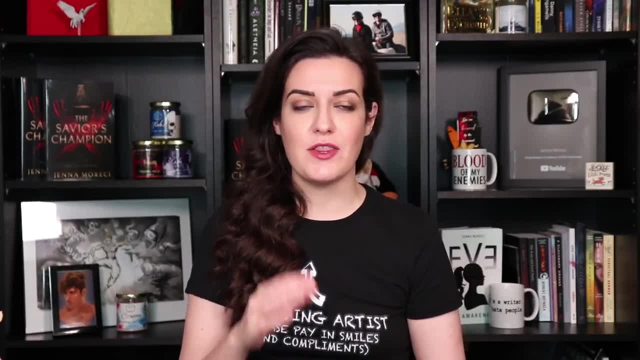 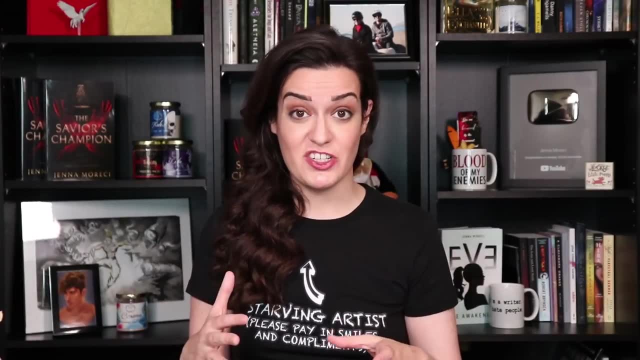 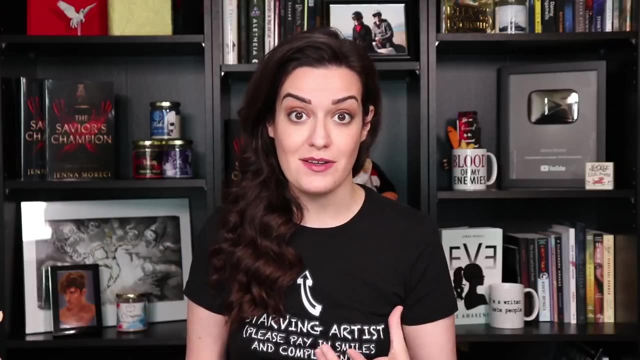 Bottom line. The reader needs to see a struggle either before or after the decision is made. Maybe they feel guilty afterward or maybe they're apprehensive to take the plunge. That's not to say that every single less-than-pure act needs to require shame or a meltdown If they're remorseful. 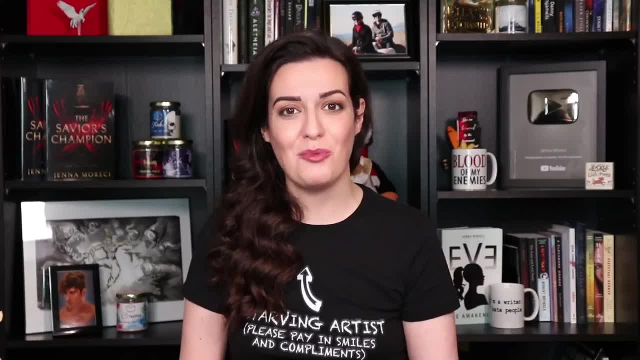 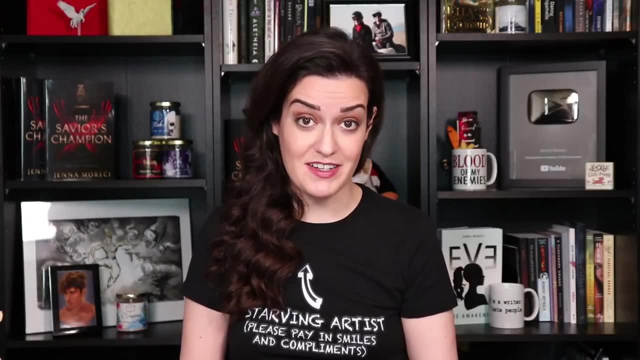 about every little thing. they're just gonna look like a big ol' wimp and that's embarrassing. But they should give a shit about the big things and their actions should have consequences when relevant. The second point is that certain lines cannot be crossed, because once you do so, you're.